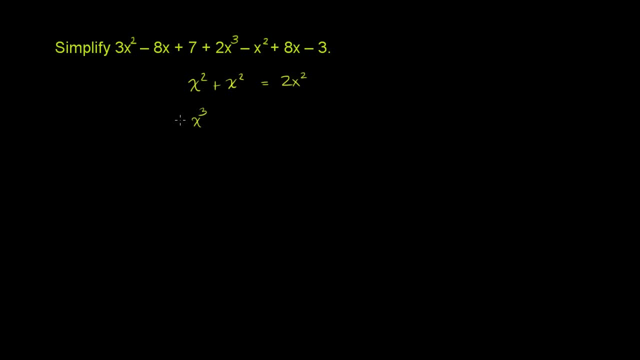 This is 2x squared. If I have an x to the third, let's say I have 3x to the thirds plus another 4x to the thirds. Well, that means I have 7x to the thirds. I can't take an x squared and add it to an x to the third. 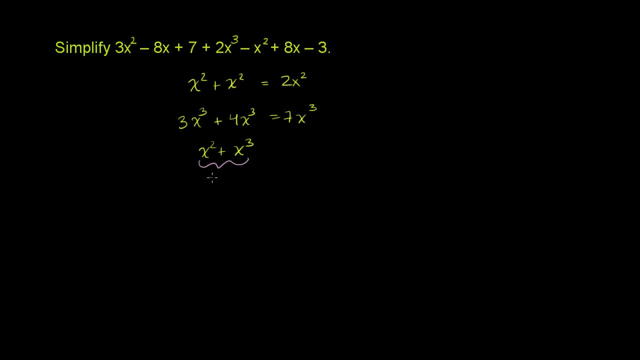 I cannot simplify this in any way. So this you cannot simplify, Cannot simplify. These are not like terms just because they both have x's. The x's are not like terms, They are not to the same degree. So, with that in mind, let's look at the x's that are to the same degree. 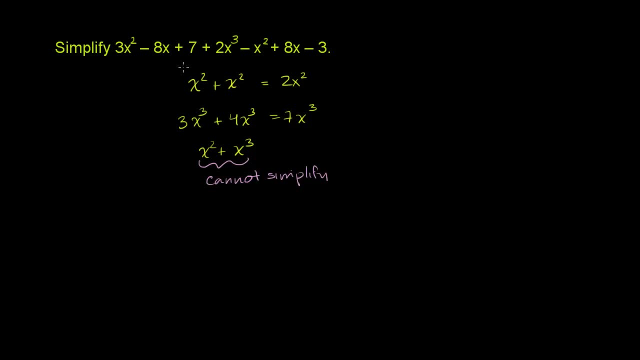 Let's start with the highest degree. So the highest degree or the highest exponent on an x here is actually this x to the third here, But it looks like the only one. It's the only place where we're raising x to the third power. 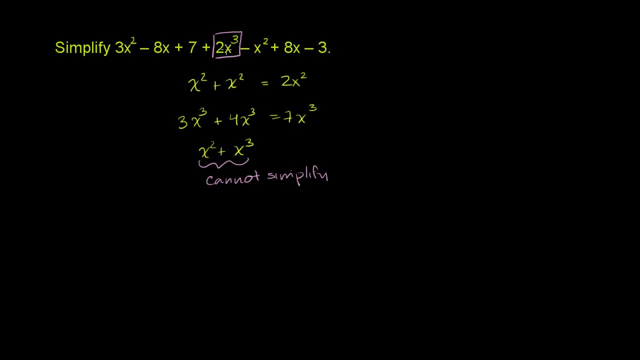 So that can't be merged or added to or subtracted to anything else. So let's just write that down. So we have the 2x to the third, And then let's look at the x squared terms. We have 3x squared terms. 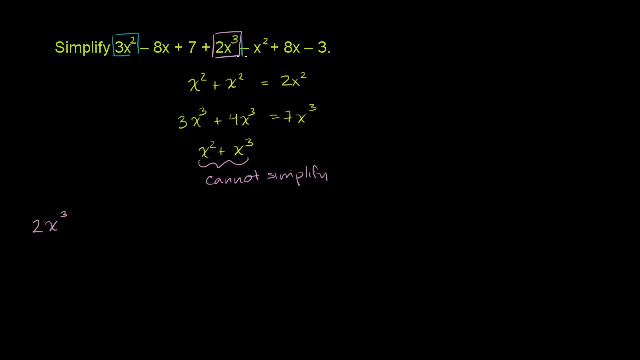 We have 3x squared over there, And then we have a minus, We have a- or we could view it as a negative x squared over there. So if we want to simplify it, we can add these two terms We can add. let me just write it down: 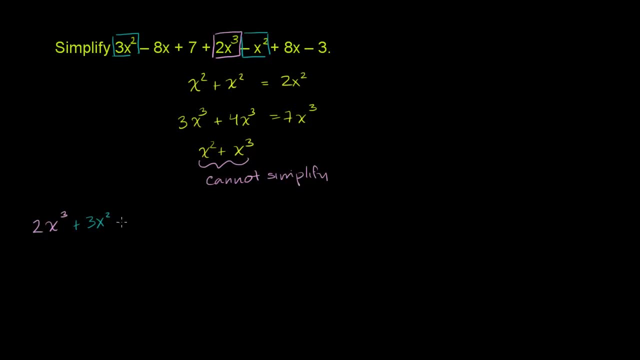 So we can add 3x squared to negative x squared. So I'm just rearranging it really right now, But I'm putting the like terms next to each other, So it will be easy to simplify. Now let's worry about just the x to the first terms or just the x terms. 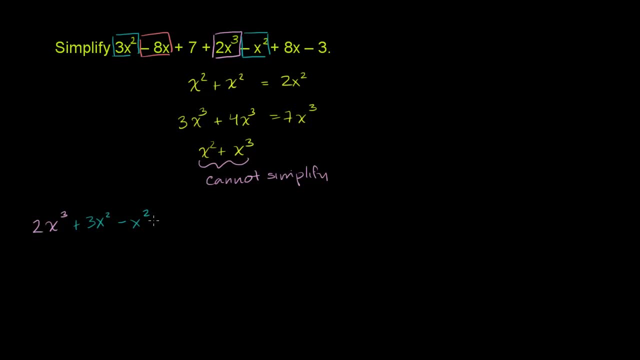 So you have a negative 8x term Right over here, So let me write it over here: Negative 8x. And then you have a positive 8x term right over here, So let me write that down. So: positive 8x. 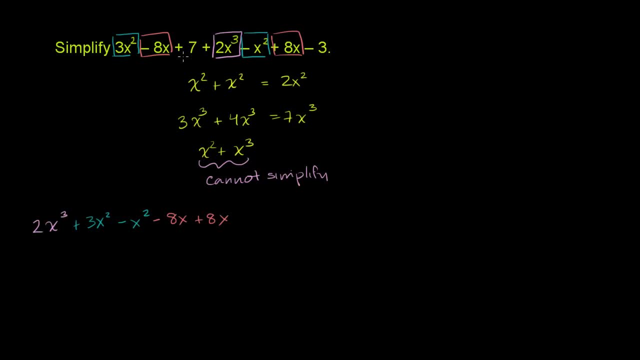 And then, finally, let's look at the constant terms. You could view those as times x to the zeroth power, And the constant terms are: you have a positive 7 over here, So plus 7.. And then you have a negative 3 over here. 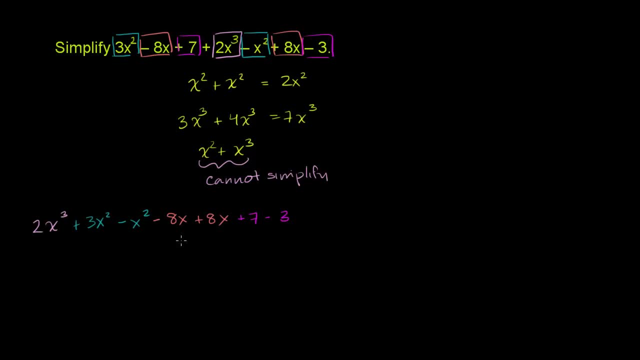 You have a negative 3.. So all I've done is I've really just used the commutative Property of addition to just to change the order or addition and subtraction, to change the order at which I'm doing this. But I've just rearranged the thing so that the like terms are next to each other.